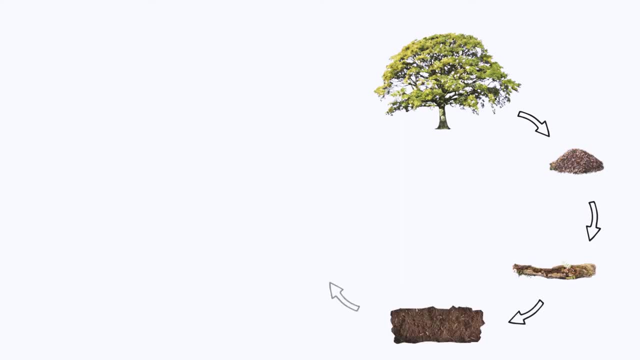 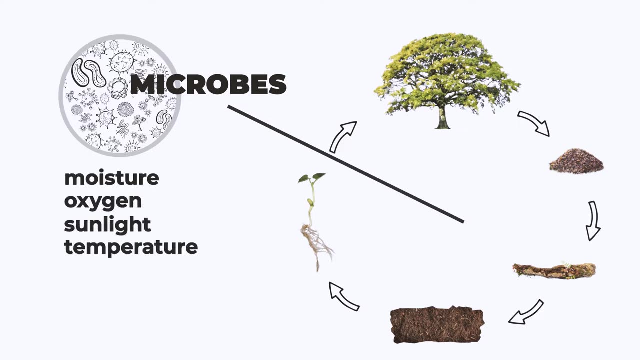 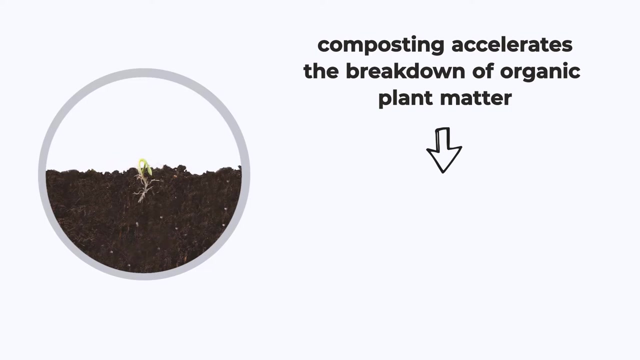 of recycling organic matter. It occurs through microbes in the soil that eat the material, But other factors like moisture, oxygen, sunlight and temperature set up the right environment for this process to occur. Composting accelerates the breakdown of organic matter into essential nutrients that form a nutritious substrate for plants to grow. Sunlight: 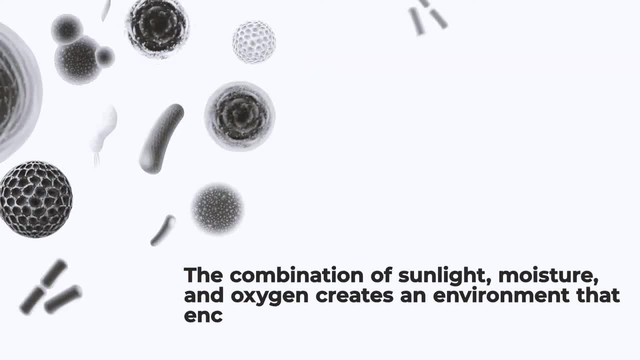 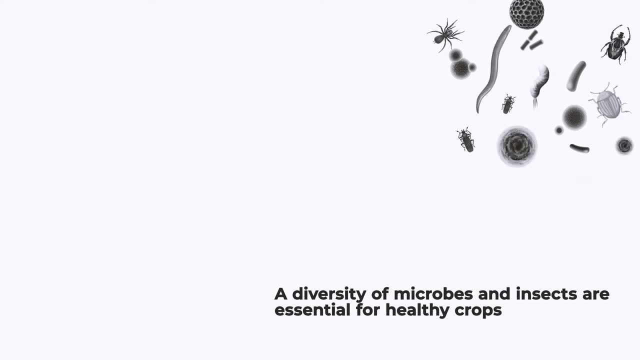 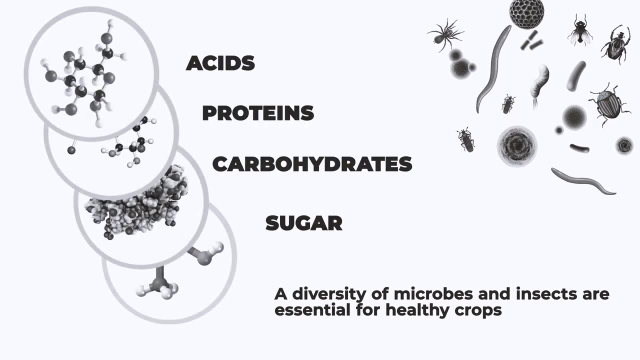 moisture and oxygen creates an environment that encourages microorganisms to multiply. A diversity of microbes and insects are essential for healthy crops. As the microorganisms eat the organic material, they leave acids, proteins, carbohydrates and sugars in the soil, and these are quickly utilized by developing plants. Organic acids are considered the spark. 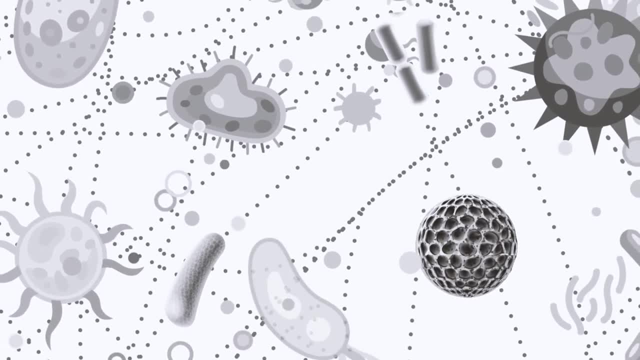 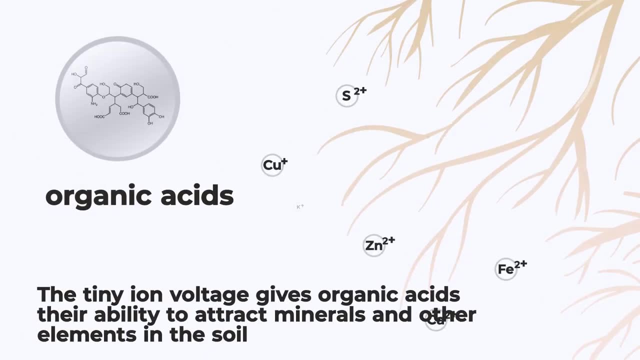 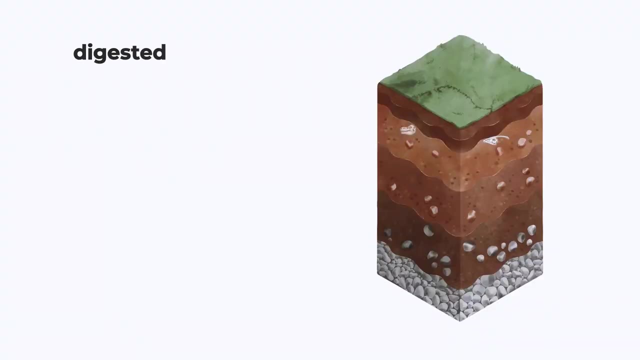 of life because they conduct electricity. For plants, this energy is in the form of organic acids. The tiny ion voltage gives organic acids their ability to attract minerals and other elements in the soil that plants can access through their root system. Decomposed organic plant material can also be used to produce organic matter. Composting is the natural process. 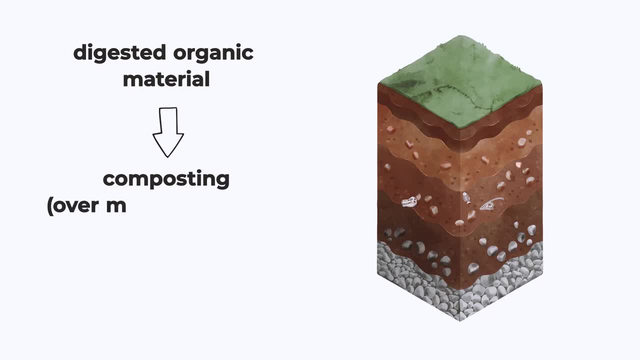 of growing organic matter. The organic matter that is used to produce organic matter becomes compost And then, if left undisturbed over millions of years, they eventually form into a humate. A humate is the final stage of mature compost. Time and weather are the greatest factors. 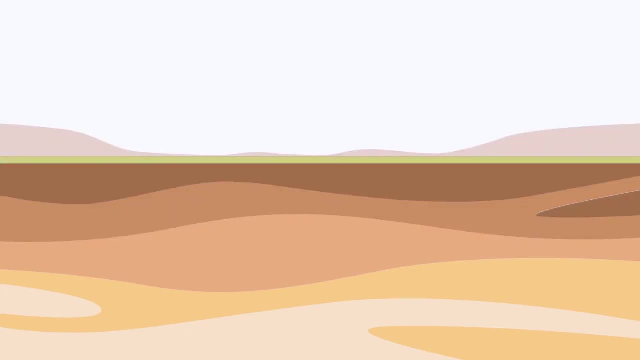 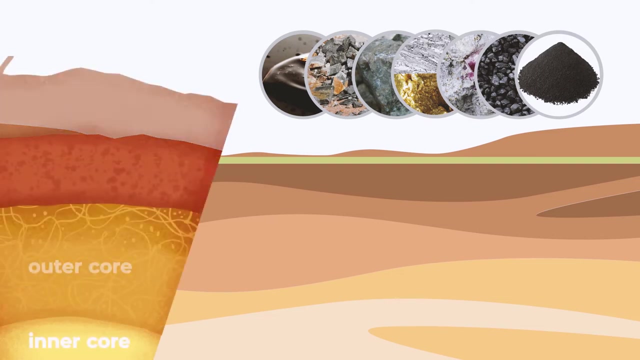 in changing the molecular structure of our soils into Earth's major deposits that we know today, like fossil fuels, metals and mineral deposits, gold, silver, crystals and rare gems, coal deposits and humate deposits. Virtually any element or mineral we mine today was created millions of years ago during the formation of our 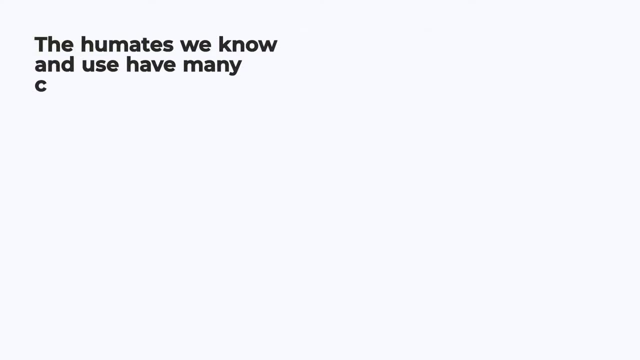 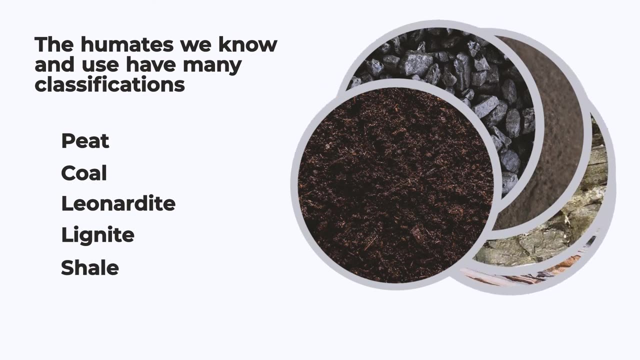 Earth. The humates we know and use have many classifications, such as peat, coal, lenardite, lignite, some types of shale and clay deposits, as well as exudate from the Himalayan mountain range. These humate substances are all millions of years old. 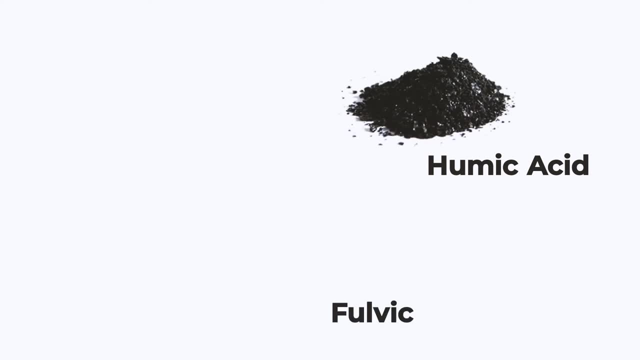 This is where humates like humic acid and fulvic acid come into play. There are several sources of humates in the world. All have different characteristics depending upon where they originate and how old they are. Humates carry ancient plant molecules known as phytochemicals.